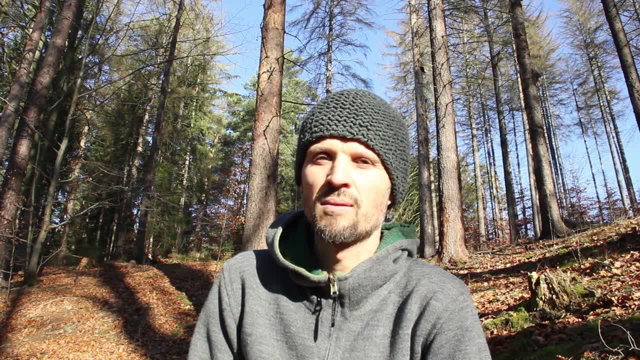 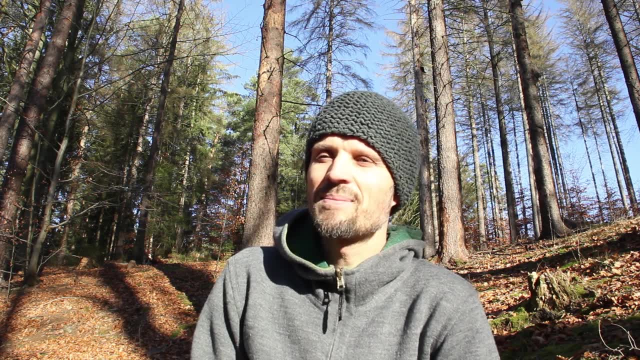 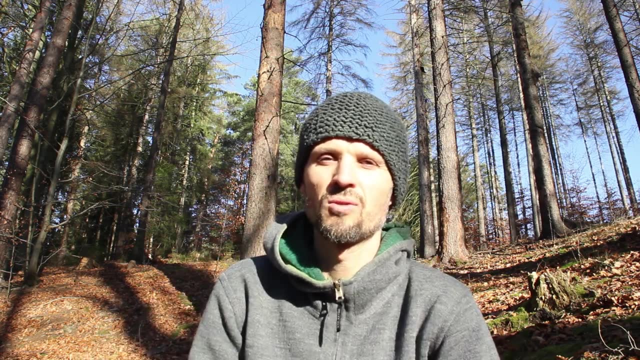 so you already have a finite subset of your theory. that's unsatisfiable. Very easy consequence of the completeness theorem, The compactness theorem. you should view it as follows: You should view it as a way to construct structures. So you have to construct. 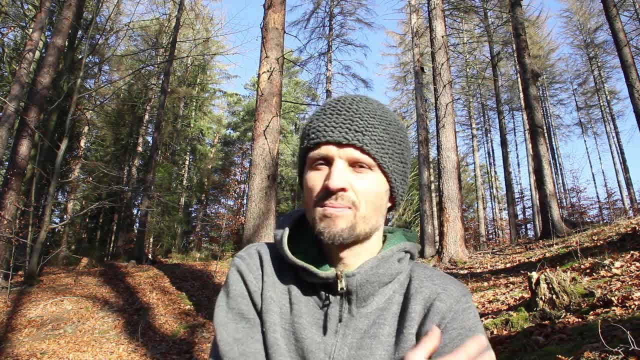 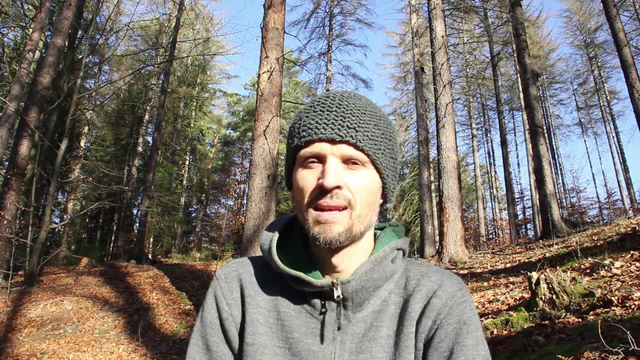 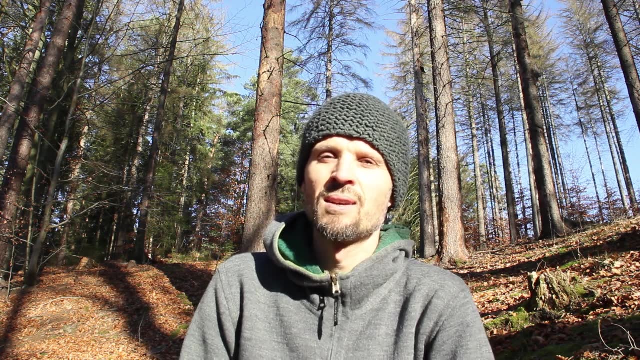 some structure, and so what you do is you write down in a big first-order theory all the properties that you want your structure to have. This will be a big first-order theory, and then all that you have to do to prove the existence of your structure is: you have to prove. 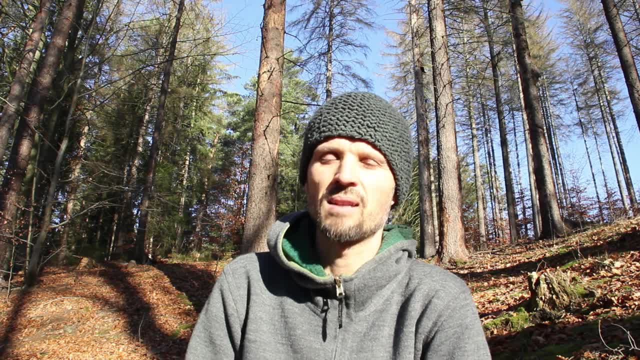 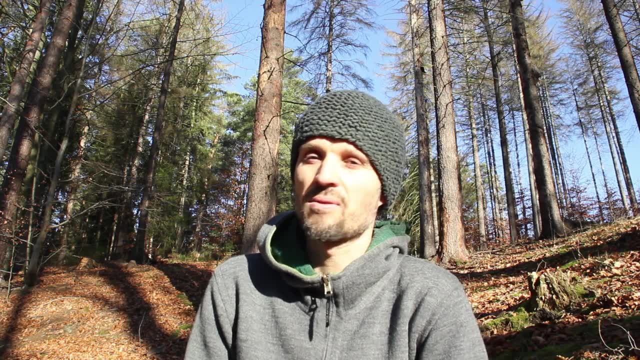 that every finite subset of your theory is satisfiable. This may be easier- Maybe you know it already- And then, if every finite subset of the theory is satisfiable, the whole theory is satisfiable and it has a model, and this is maybe the model you wanted. 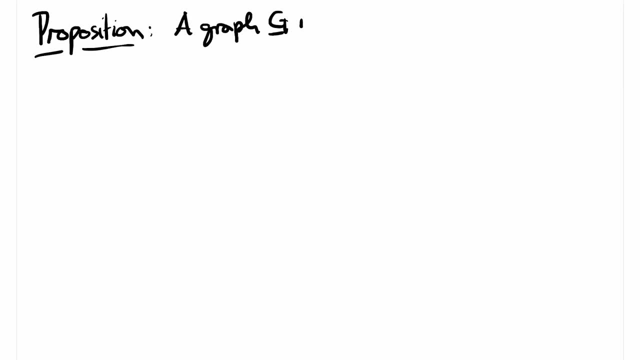 A standard application of the compactness theorem is the statement that a graph, G, is k-colorable if, and only if, every finite subgraph of the graph is k-colorable. For the interesting direction of the proof, suppose that every finite subgraph of G is k-colorable. To prove that G is k-colorable. 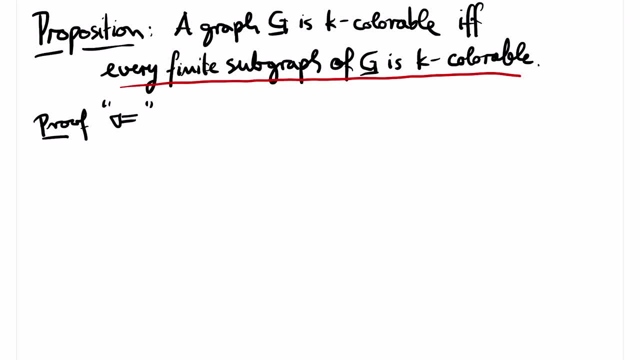 we first write down a first-order, The first-order theory that corresponds to the k-colorability of the graph G. The signature of this theory is a binary relation for the edges of G and a constant symbol, cv, for every vertex v of the graph G. And finally we use k-unary. 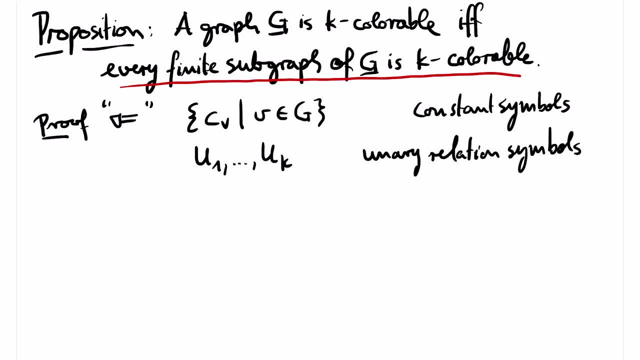 relations u1, u2 and so on, until uk to represent the color classes. t consists of the k-unary relation u1, u2 and so on, until uk to represent the color classes. This consists of the following sentences: First of all, we have the sentence that there is an edge between cu and cv. 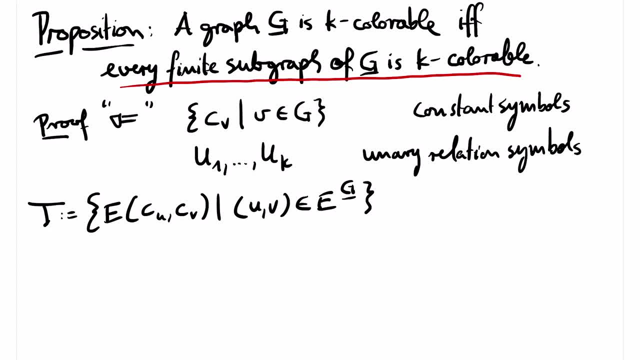 if u and v form an edge in G, Then we have the sentence that states that every vertex is contained in at least one color class. Finally, we have the sentence that if the same color class contains x and y, then there should not be an edge. 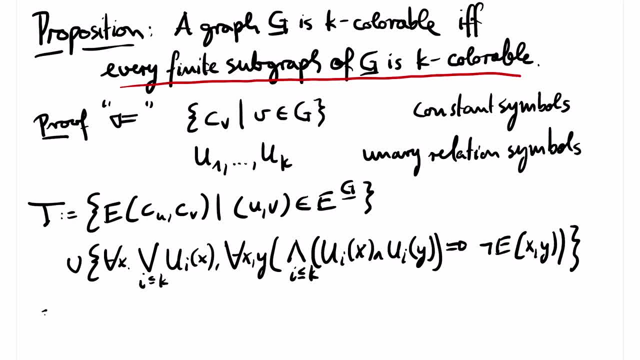 We claim that every finite subset of this theory, t, is satisfiable. Let f be a finite subset of t. Only finitely many constant symbols can appear in f. The respective vertices of G for these constants induce a finite subgraph, h. By assumption h is k-colorable. 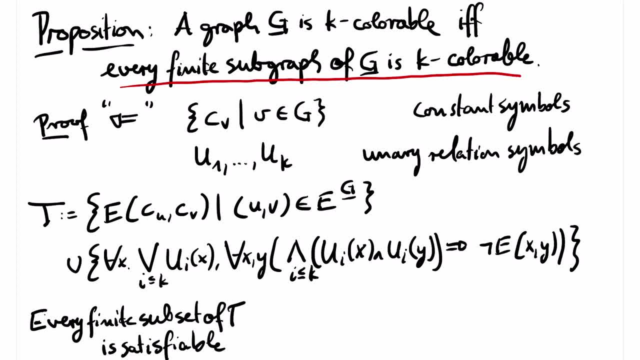 We then set u to be the color class of the color i. with respect to this coloring, The expression of h by constant symbols and the unary relations I just defined is a model of f. The compactness theorem therefore implies that t has a model. 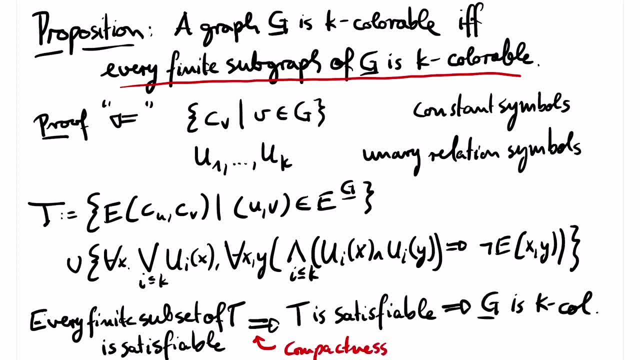 We can use this model to define a k-coloring of G as follows. If cu is in ui in the model, Then we color the vertex u of g by the color i. It's straightforward to verify that this gives a proper k-coloring of g. 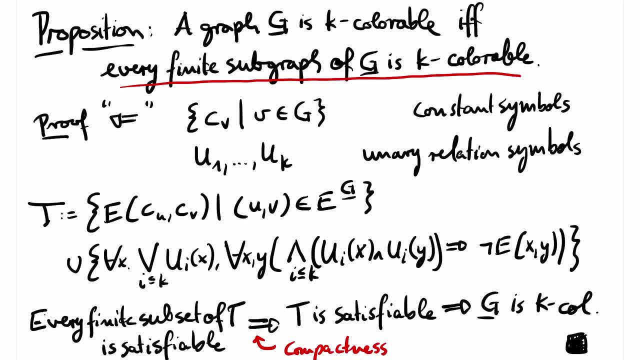 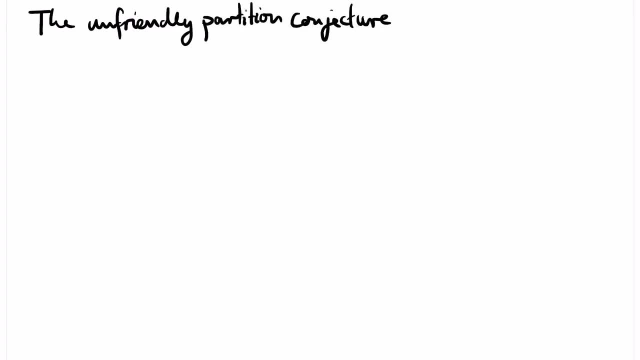 We have to be careful with applications of the compactness theorem. There are some statements that almost look like statements that could follow from compactness, but they don't. There's, for example, the so-called unfriendly partition conjecture. We start with the observation that every finite graph has a so-called unfriendly partition. 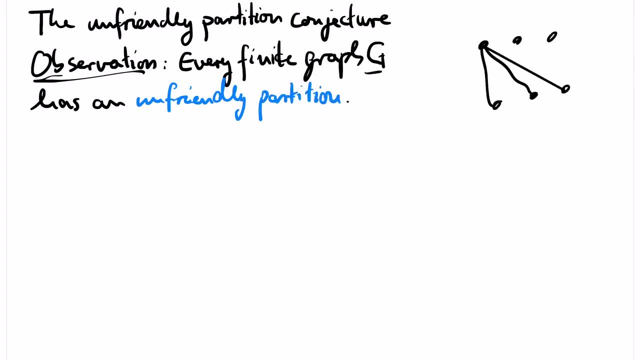 This is a partition of the vertices such that every vertex has at most as many neighbors in its own part than it has neighbors in the other part. Let's have a look at the following example drawn on the right. It has, for example, the unfriendly partition into blue and non-blue vertices. 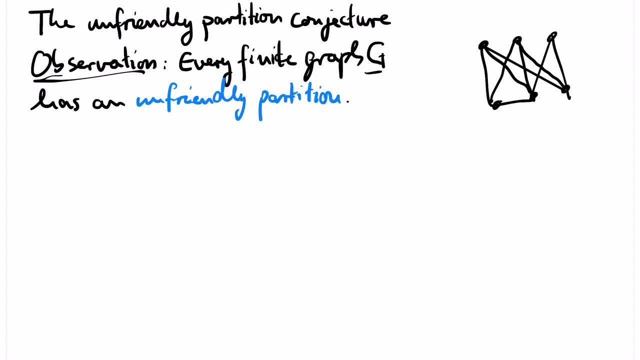 In fact, it is easy to construct unfriendly partitions greedily. Just start with any partition. If it has a vertex which has more neighbors in its own class than in the other class, push it over to the other side And repeat. In this way, the number of edges between the two parts increases properly strictly. 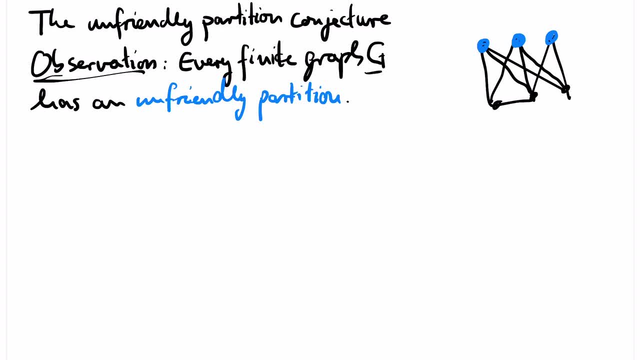 In a finite graph, this can only happen a finite number of times, So eventually we reach an unfriendly partition. Our greedy approach even leads to an algorithm to construct unfriendly partitions. Now let's have a look at arbitrary graphs. We already know that every finite subgraph has an unfriendly partition. 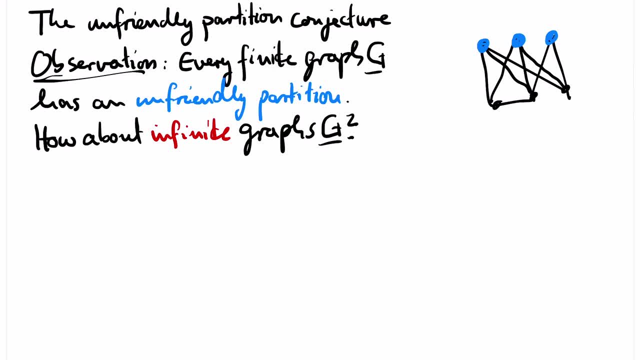 So we are tempted to conclude that G has an unfriendly partition, But this is false. Schellach and Milner constructed a graph with uncountably many vertices without an unfriendly partition. The same question for countable graphs is open, And this is the unfriendly partition conjecture. 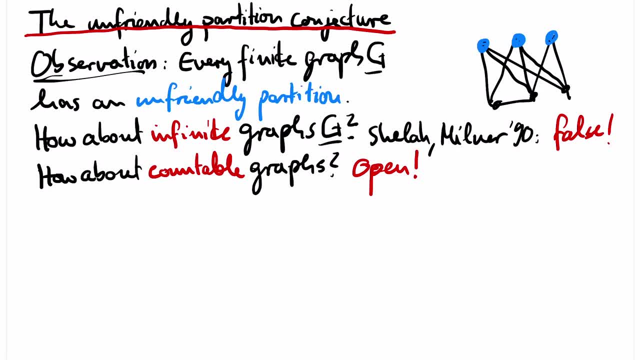 So why can't we apply the compactness theorem here? Well, in order to apply the compactness theorem, we need a first-order theory. And what should this first-order theory be? What can be shown using the compactness theorem is that the statement is true. 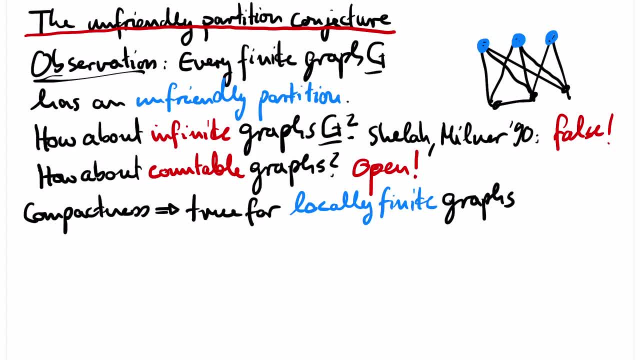 for graphs that are locally finite. For graphs where every vertex has only finitely many neighbors. Again, we work with a signature to show this. that contains a constant symbol cv for every vertex v. That contains a constant symbol cv for every vertex v. 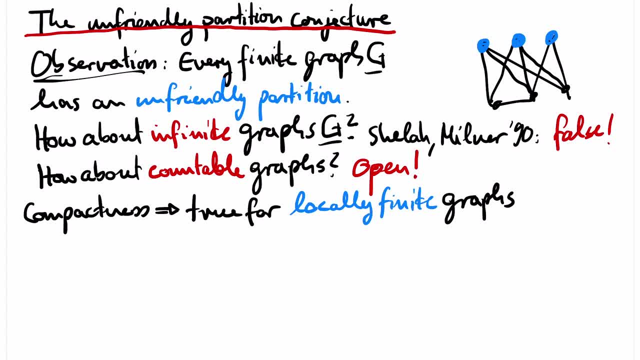 That contains a constant symbol cv for every vertex v Of the graph. We also need a unary relation symbol p that denotes one of the parts of the partition. To express that p and not p define an unfriendly partition, we use the following first-order sentence: phi u n. 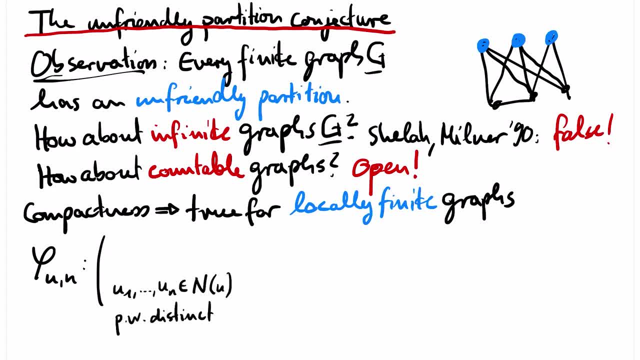 It states that if there are pairwise distinct neighbors u1 up to u, n of u in G and all of them are in p, then they are also n. Then there are also n pairwise distinct neighbors v1 up to vn of u in G that are all outside of p. 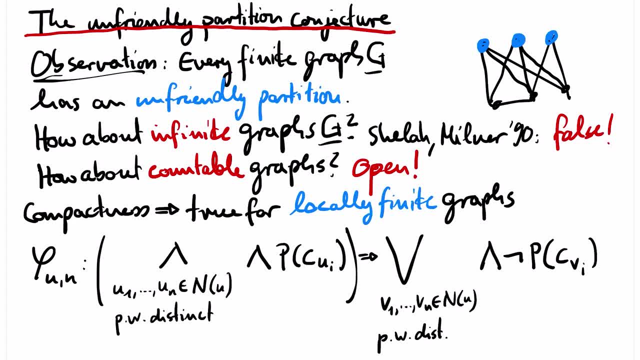 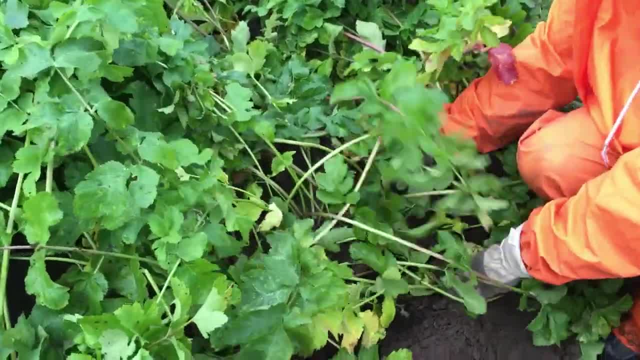 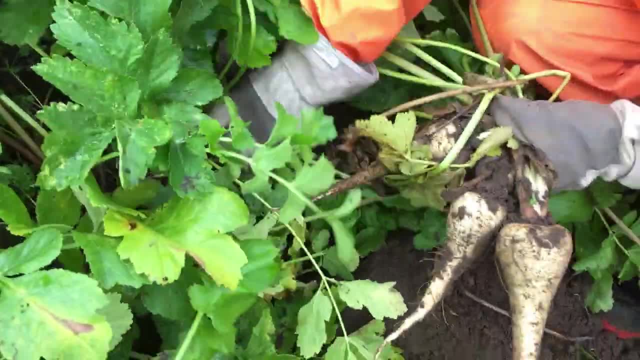 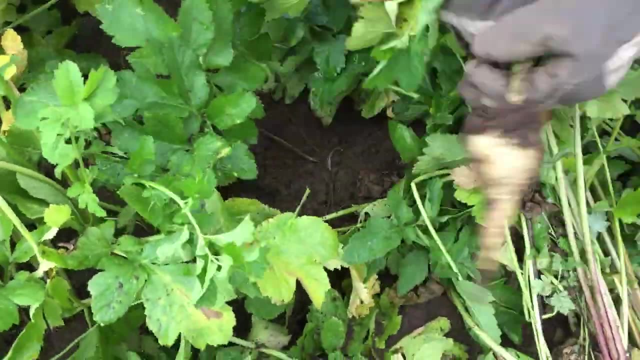 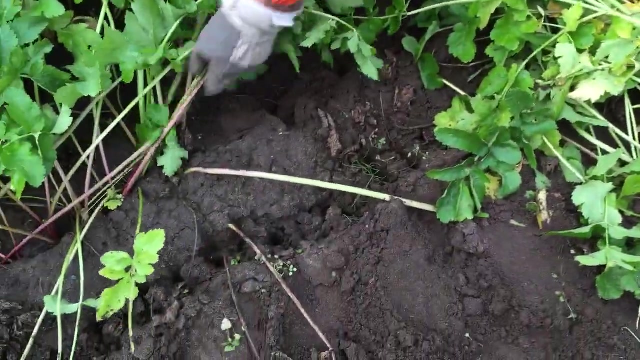 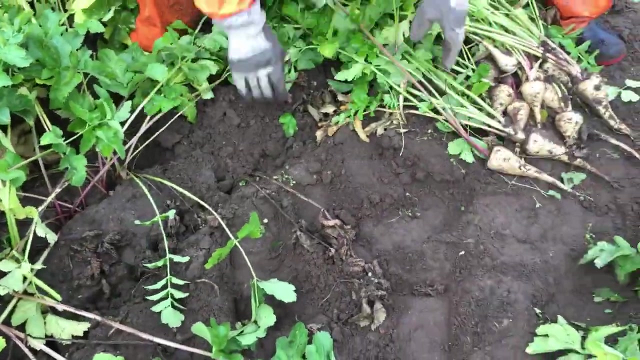 Then there are also n pairwise distinct neighbors, v1 up to vn of u in G that are all outside of p. The remaining argument is left to the audience. The remaining argument is left to the audience. The remaining argument is left to the audience. 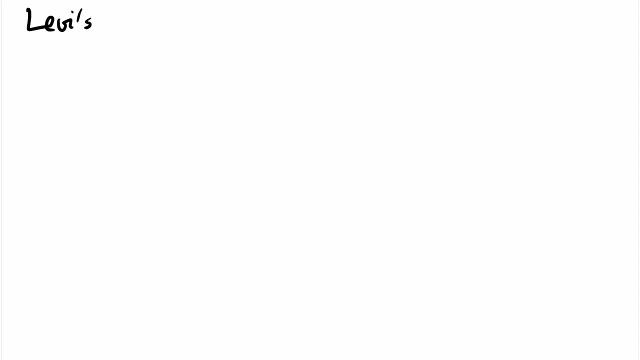 We have seen two applications of the compactness theorem for graphs. We will now also present an algebraic application of the compactness theorem. 폭수, Turin, pmdln, рв, llupλ, Ku2, R, AU. patriq Jr, 80MmrPe, hal. 2.0.3iHZ2, csq, p1.0.1i, mрnJ, op-, rvAl, Имx& ko m div2, sch. 0x264a, ,162p, 0.com. here also. 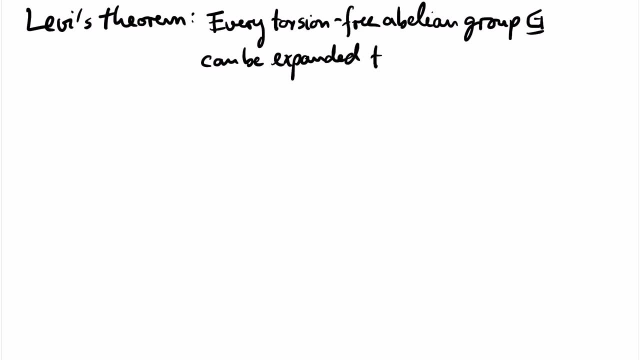 theorem for groups, and we will prove levy's theorem. every torsion free abelian group g can be expanded to an ordered group. note that the axioms of ordered groups are first order sentences and that the property to be torsion free is a first order property too, and in fact all sentences. 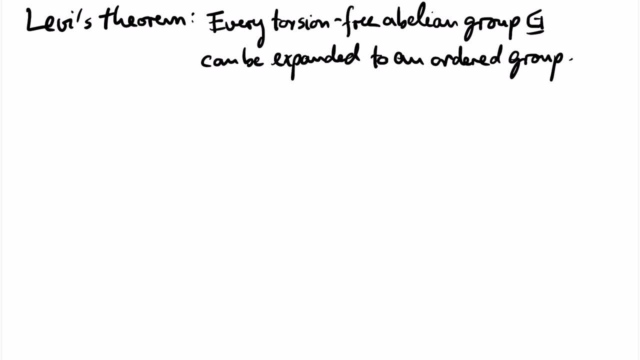 can be chosen to be universal, that is, we only need universal quantifiers applied to some quantifier free formula. so let t be the first order theory of ordered abelian groups. let s be the theory of the expansion of g by constants for each element of g. we claim that for every finite 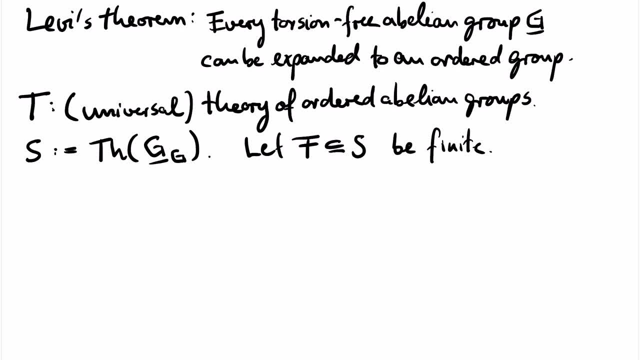 subset f of s. the union of f and t is satisfiable only finitely. many constant symbols can be quantified for each element of g, so let t be the first order. theory of ordered abelian groups can appear in f. let h be the subgroup of g that is generated by these constants. 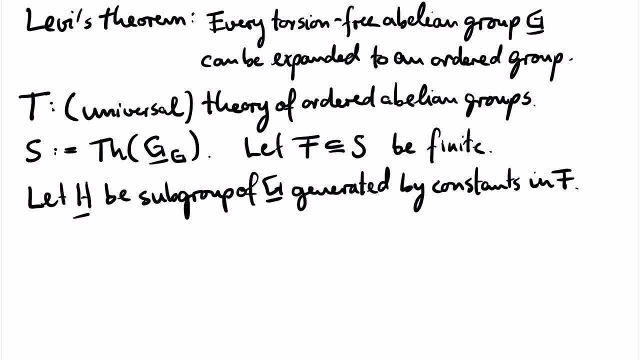 then h is a finitely generated abelian group, and abelian finitely generated groups are classified by the fundamental theorem for finitely generated abelian groups. we know precisely how they look like. so we look in the list and we see that if h is torsion free, it must be of the form z to the n. 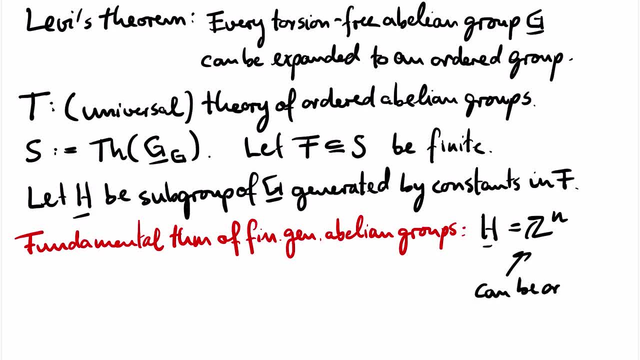 and z to the n can be linearly ordered, for example by the lexicographic order. this shows that the union of f and t is satisfiable. therefore, the compactness theorem implies that the union of s and t is satisfiable as a model. let's call it m. the constants in the signature induce a substructure of m with the same 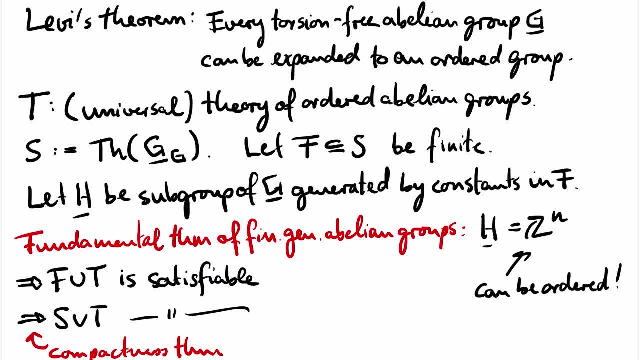 domain as g is the constant in the signature and uses substructure of m with the same domain as g, And as the axioms of T are universal, they also hold in this substructure. So the reduct of the substructure with the signature of ordered abelian groups is an ordered abelian group. 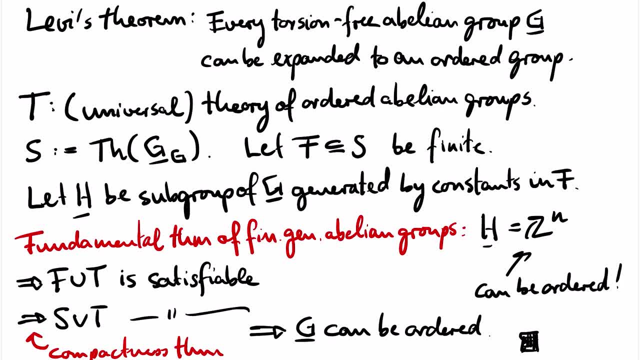 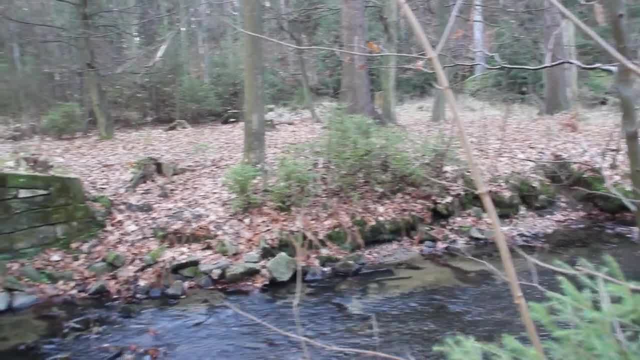 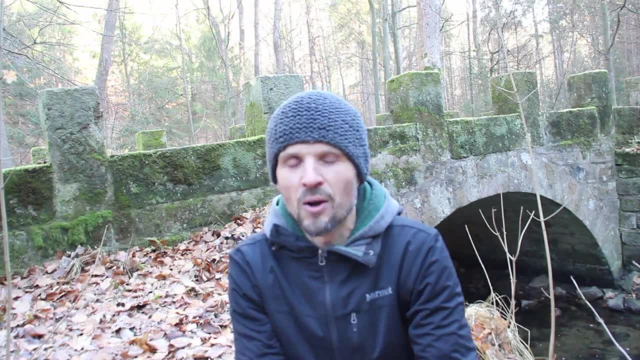 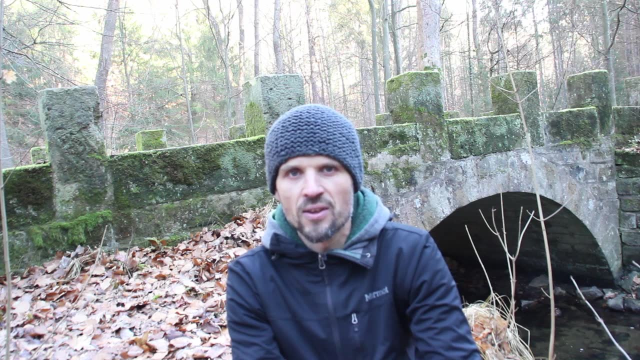 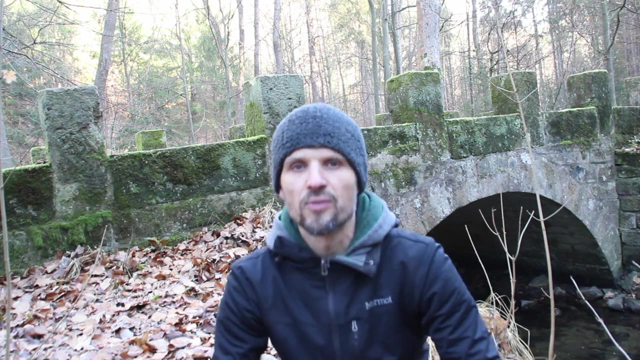 And it expands G. so we found an ordered group expansion of G. The compactness theorem can be used to show something about the limits of first-order logic, To prove that certain things cannot be expressed in first-order logic. For example, one can show easily- we'll see it later- that there is no first-order theory that would axiomatize precisely the class of connected graphs. 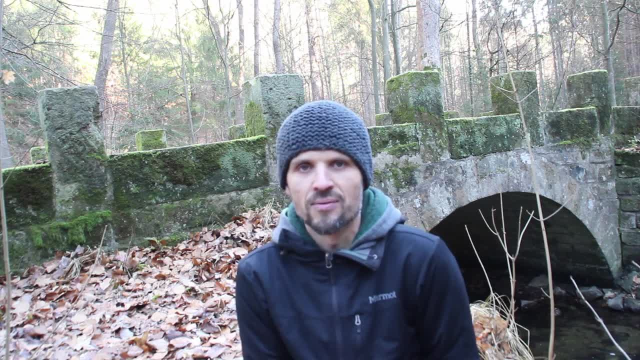 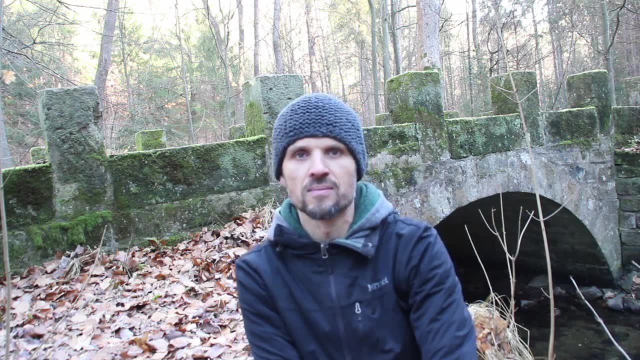 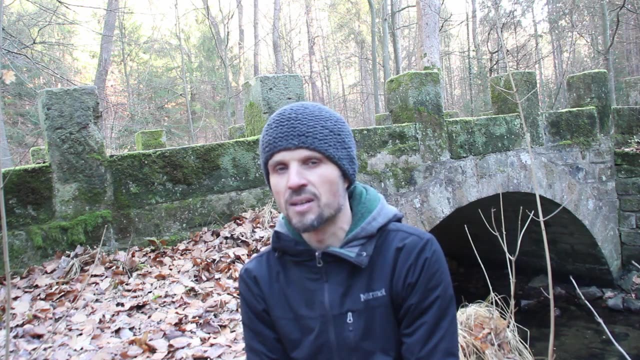 So actually it's a common topic in computer science to make first-order logic stronger, To add something to first-order, Because it can't even express connectivity of graphs, which is something we would like to express with a logic. So you add something to first-order logic, but it turns out that as soon as you add a little bit to first-order logic you lose the compactness theorem. 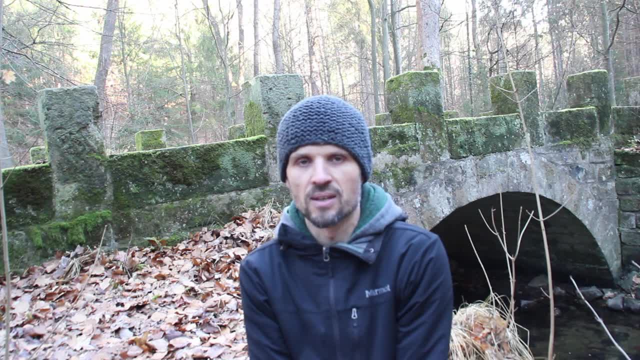 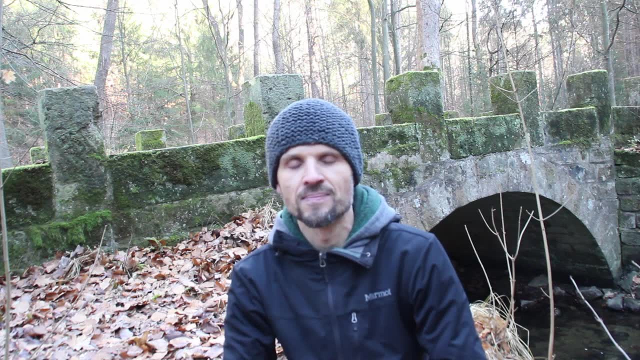 And that's maybe one of the justifications of first-order logic. We like first-order logic because it has the compactness theorem, Something so nice, And it's a common thing, And it's a common thing That we would like to have it. 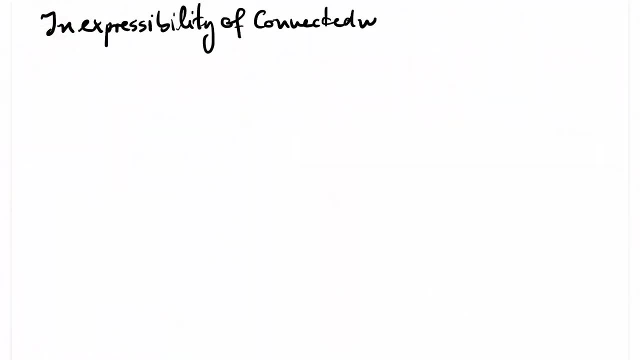 First-order logic can't express connectivity of graphs Formally. the claim is that there is no first-order theory T, whose models are precisely the connected graphs. To prove this, let C and D be two constant symbols. Let phi sub n be the sentence that expresses that there is no path of length. 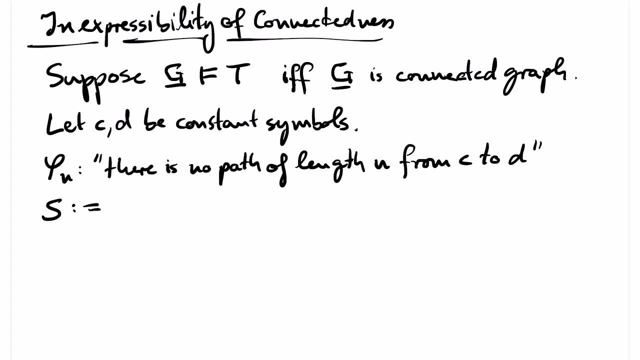 N from C to D, Let S be the set of phi, n for all natural numbers, n. Then unions of T with finite subsets of S are satisfiable Because there are connected graphs with vertices at arbitrarily large distance. Hence, by compactness, T union S is satisfiable. 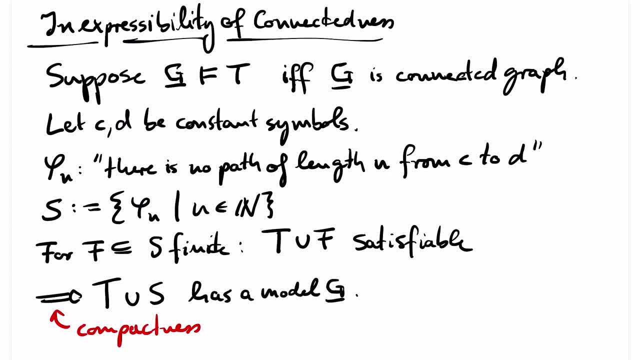 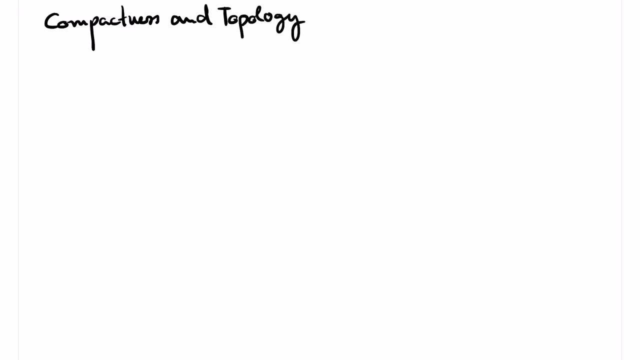 It has a model G. Since G satisfies S, there is no path from C to D in G And this is a contradiction to the assumption that the models of T are connected. You know the name: compactness from topology. A topological space is compact if every open cover of the entire space contains a finite subcover. 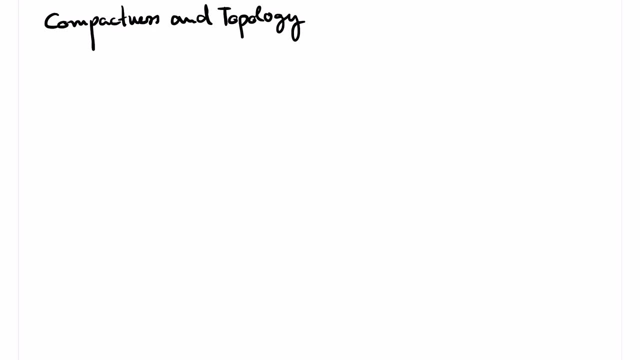 This looks similar to the compactness theorem of first-order logic. Can we make the similarity precise? We would like to define a topology such that the topological space contains a finite subcover. Instead, the compactness theorem translates to the statement that the topology we defined is compact. 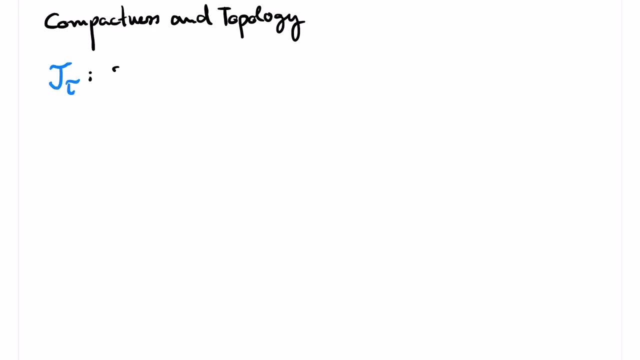 And this is indeed possible. Our topological space is the set of all complete tau theories for some fixed signature tau. To define the topology I have to define what the basic open sets are. If phi is a first-order tau sentence, then the set T sub phi. 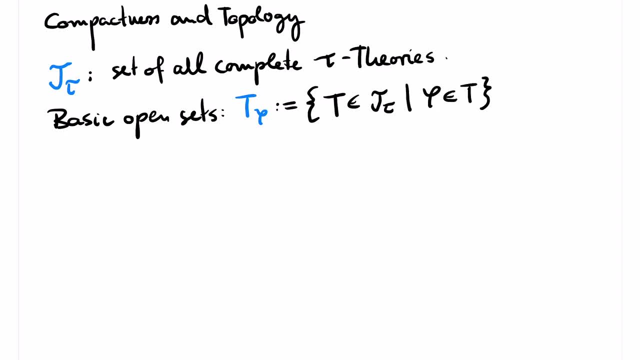 is the set T sub phi, The set of all complete theories that contain phi. Now, the basic open sets in our space are precisely the sets of the form T sub phi. It's easy to verify that this is indeed a topological space. 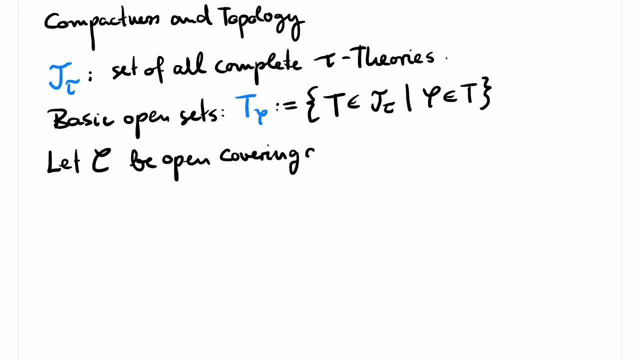 Suppose now that we have a covering of this space by open subsets, Let's call the covering C calligraphic C. We may assume that C is of the form T sub phi, where the index phi runs in the form T sub phi. 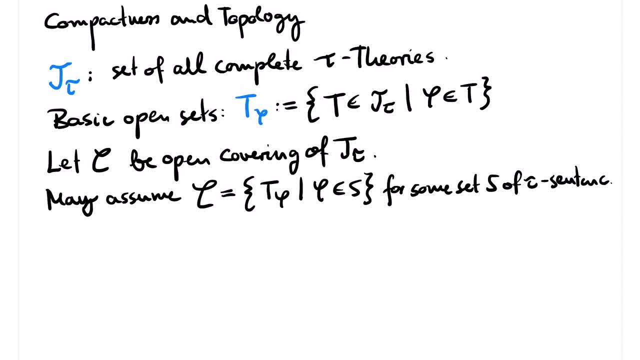 Where the index phi runs in the form T sub phi. Where the index phi runs over some set of first-order sentences, S, Let S prime be the set of all negations of sentences in S. Since C covers all complete theories, the set S prime is unsatisfiable.